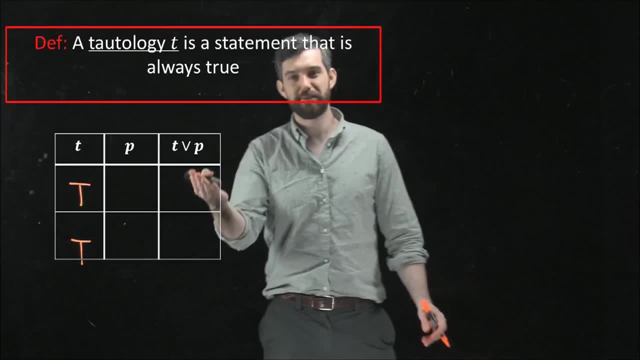 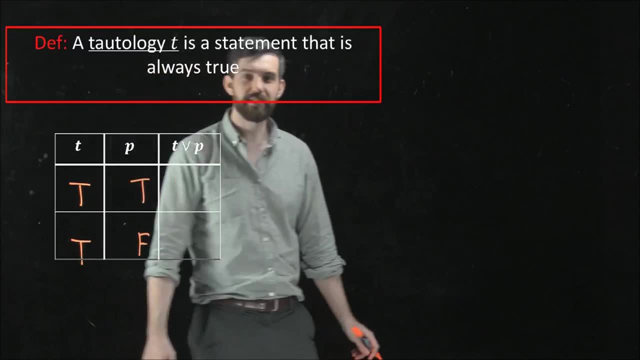 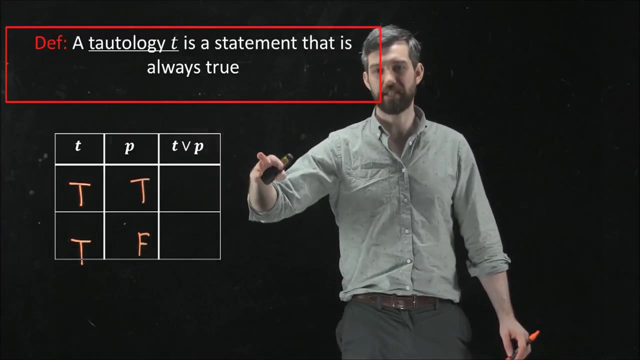 true, true, true, true, true everywhere. And then I also have this other statement, P. P is just a normal old statement here, So it can be true or false. So maybe its first possibility will be true and its second possibility will be false. And then, if I want to take a tautology or some, 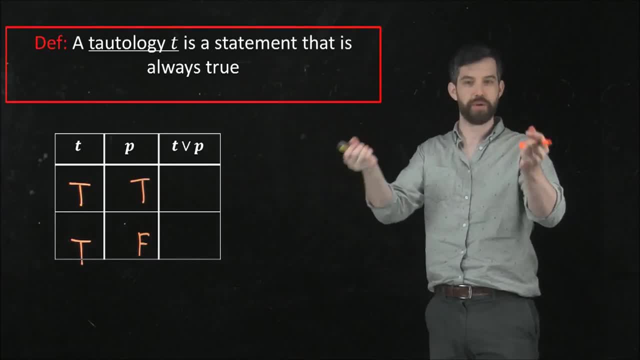 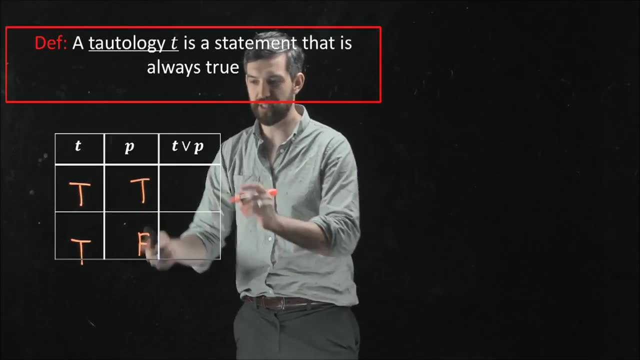 statement remember or is true if one of the two are going to be true? But the tautology is always true, So it's always the case that one of them is going to be true here. So there's two trues there. 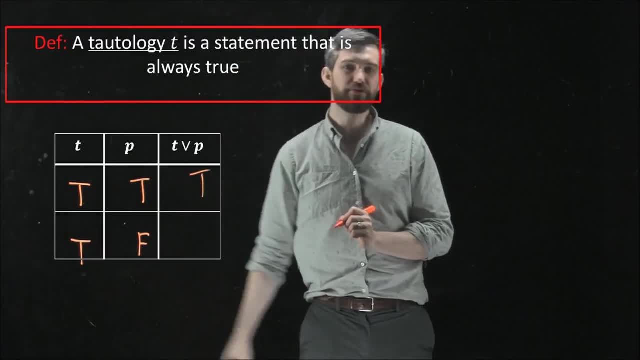 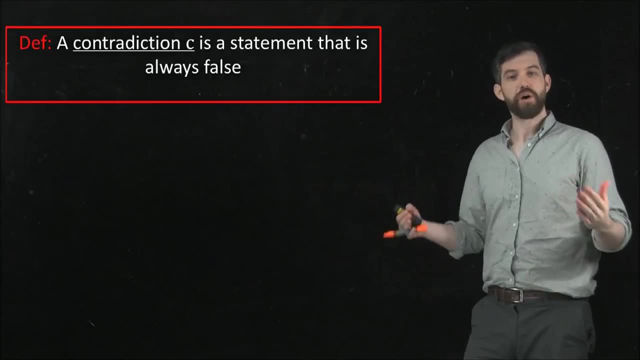 which is good enough to give me a true here. There's only one true here, but that's fine, It's an or statement. Only need one of them to be true, So that's going to be true there as well. I can. 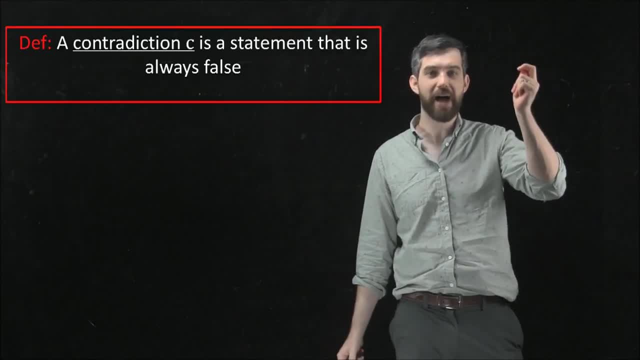 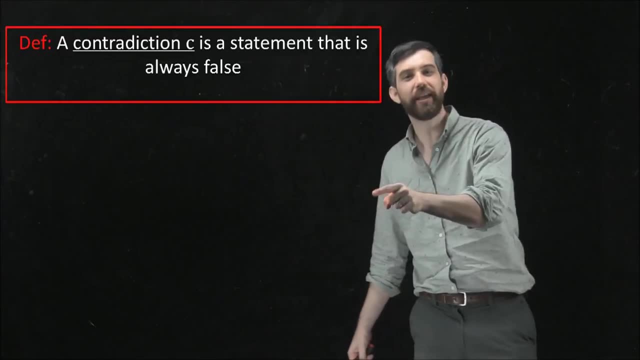 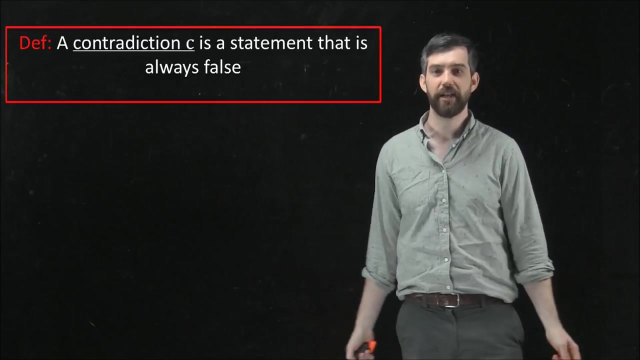 also have contradictions. Contradictions are labeled by a, C, now for contradiction, And this is another example. So this is an example that dog is a reptile. Again, in the notion of a dog it is implicit that dogs are mammals and not reptiles. So it can never be true that that 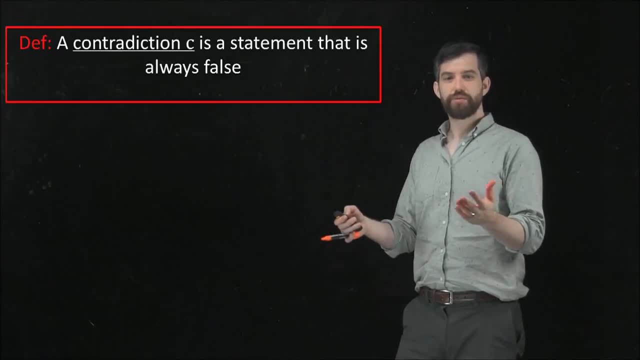 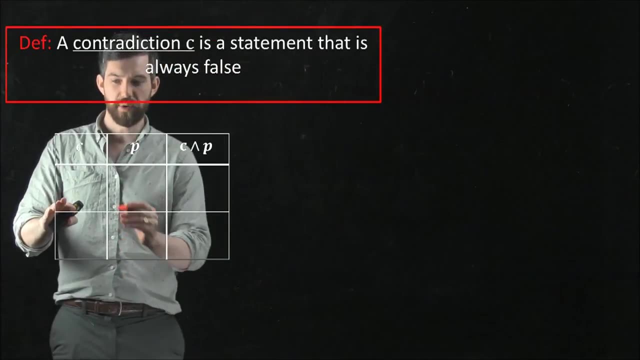 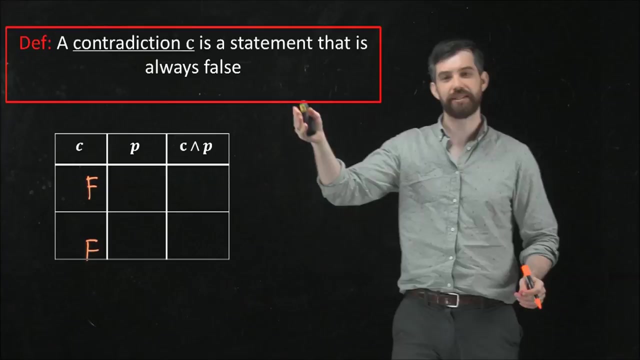 dog is a reptile. So this means that in our truth table, whenever I have a C, it is going to be a column of all falsehoods. So here I'm going to have a false, and here I'm going to have a false, And then I've also done a simple example I'm trying to look at. 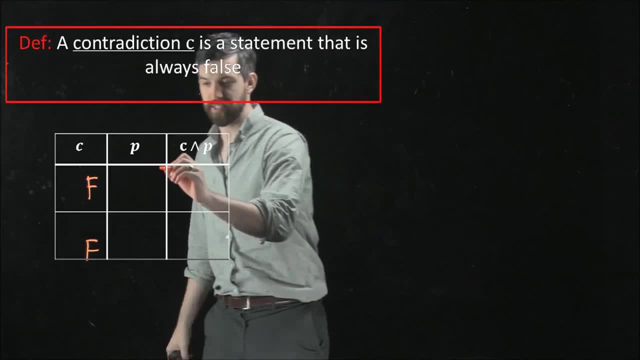 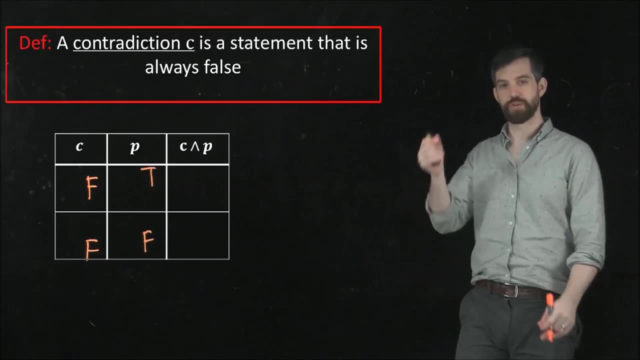 where P is just some other statement. so let's fill in a couple different possibilities for P. It could be true and it could be false. And then, if I want to look at my final conclusion, which was C and P, remember AND requires both of them to be true. 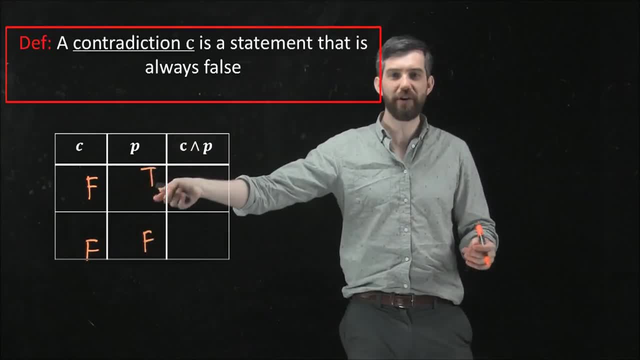 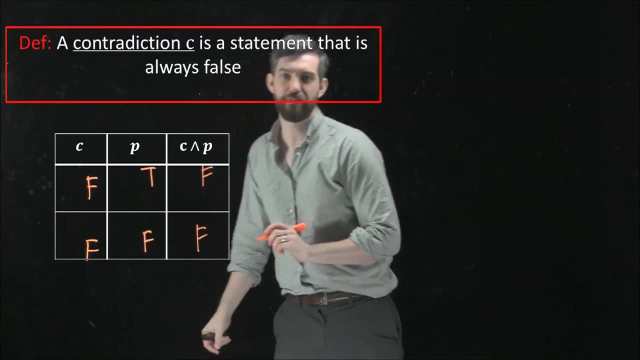 But because we have my contradiction always being false, it will never be the case that both of them are true, And so since there's one false there, there's going to be a false there. Since there's a false there, there's going to be a false there as well. 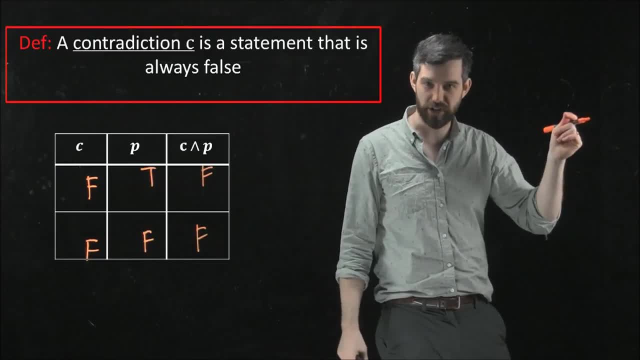 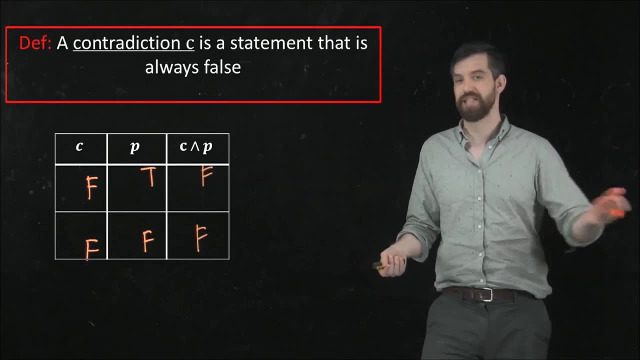 So when I had an OR statement with a tautology, it forced that to be a tautology. It made it always going to be true. If you took OR a tautology, you could just take the value of the tautology. it would be always true.